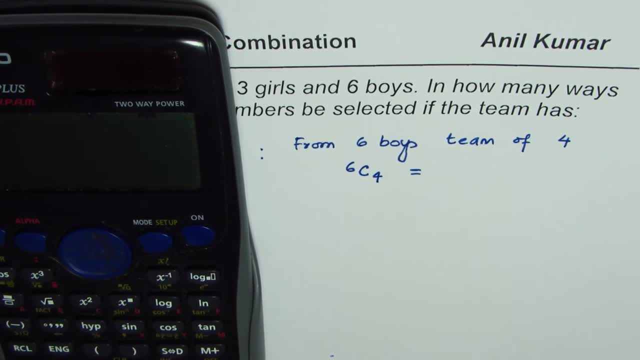 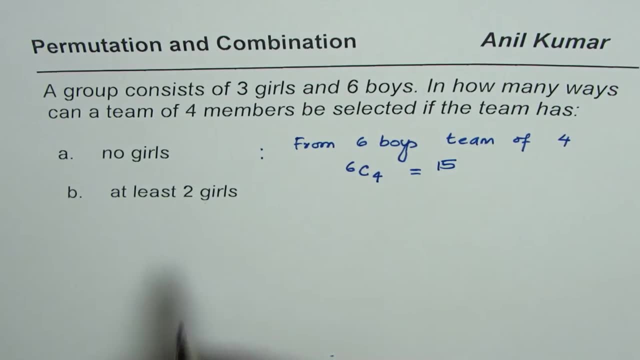 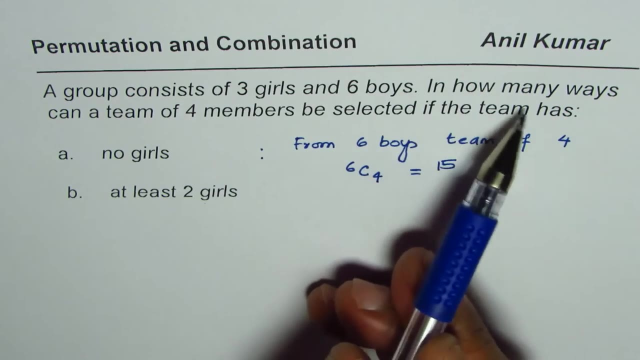 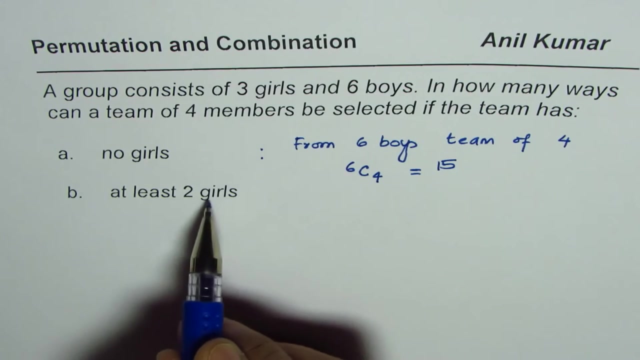 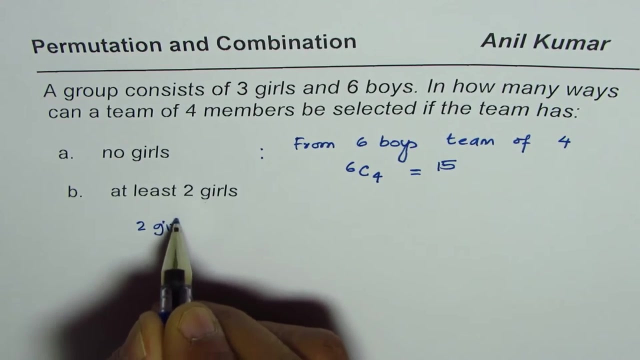 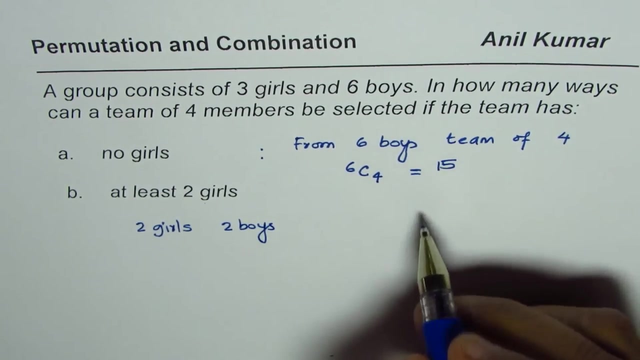 have six C4 equals to 15.. So these are 15 possible cases. Now let's do the next one. It says a group consists of three girls and six boys. In how many ways can a team of four members be selected If the team has at least two girls? Now there are three girls in all. So that means either we have two girls, right? So if you have two girls, we need a team of four. That means two girls and two boys. That is one option. The other option is we can have three girls and one boy. So these are the two different combinations. 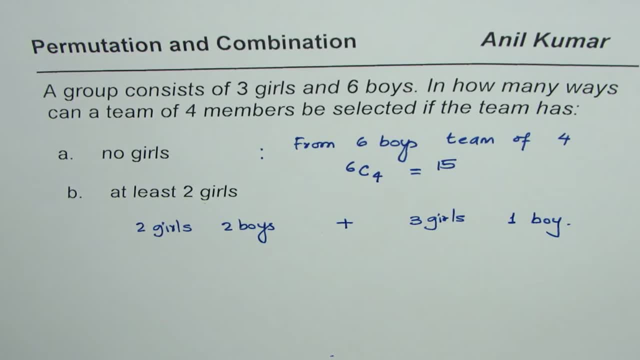 And you know we need to add them up. So that is the strategy for such questions. Now you need to select two girls out of three, So that is three C2 times two boys out of six. six C2 plus three girls out of three, That means three C3 times one boy out of six boys, six C1, right? 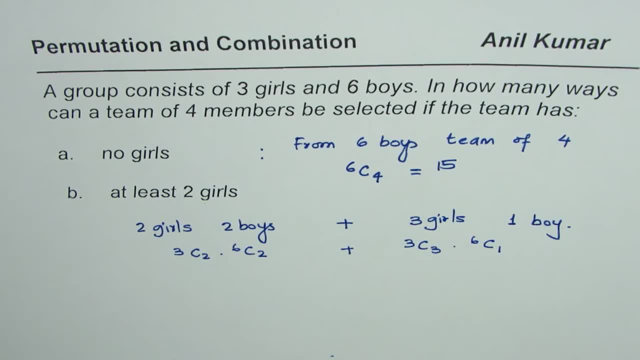 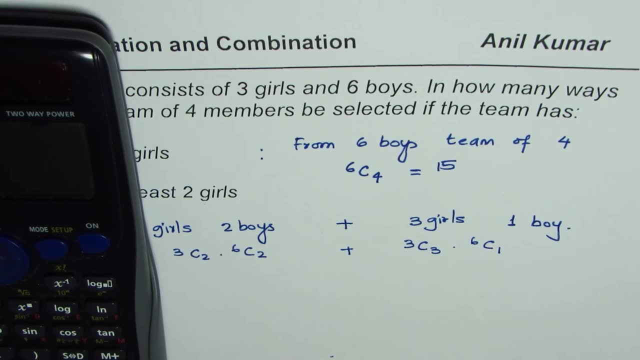 that should give you the answer right. so let's use the calculator, find the answer. so we have 3 c 2, so 3 c 2 equals to 3. so we get 3 here times 6 c 2, so 6 c 2, that is equals to 15. 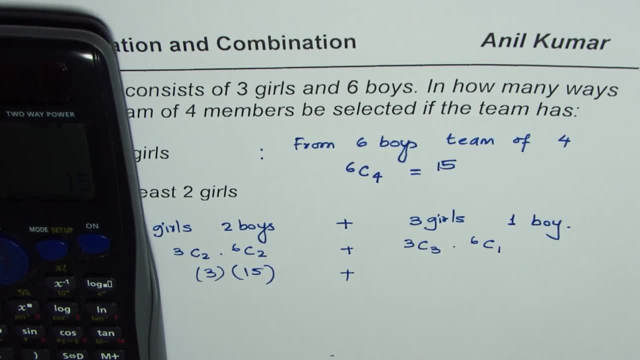 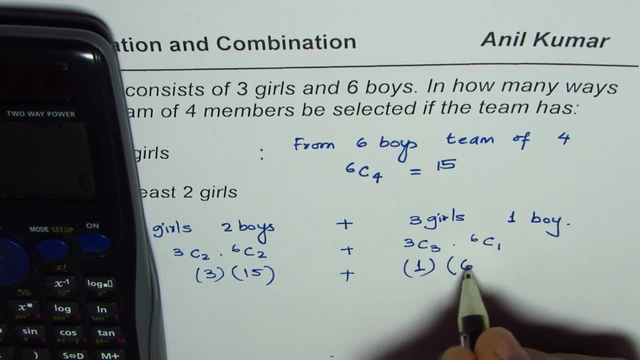 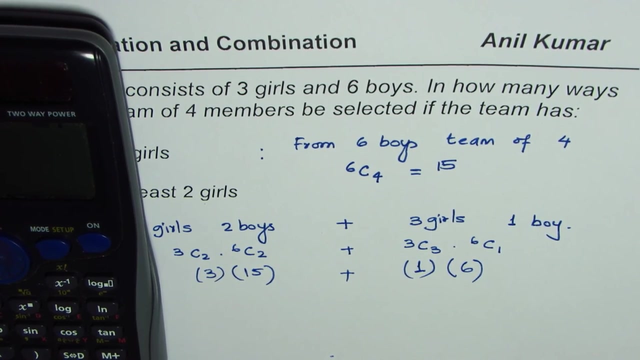 plus 3 c 3, so we have 3 c 3 equals to 1 times 6 c 1. 6 c 1, okay 6, and so we get our answer 3 times 15 plus 6, which is equals to 51. so in this particular case, 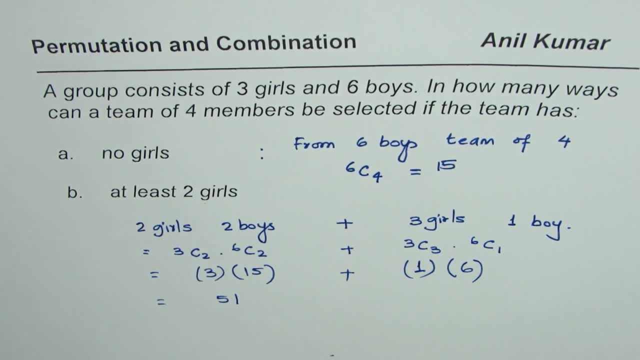 15 plus 3 c 3, so we have 3 c 3 equals to 1 times 6 c 1. 6 c 1, okay 6, and so we get our answer 3 times. the answer is 51. so so when at least two girls are there in a four-member team, then there are 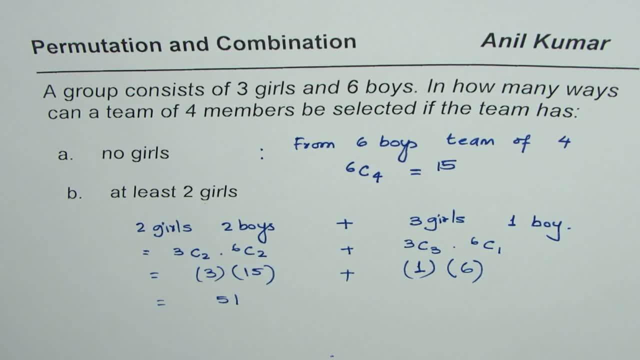 51 combinations. i hope it helps you to understand the concept. thank you and all the best.